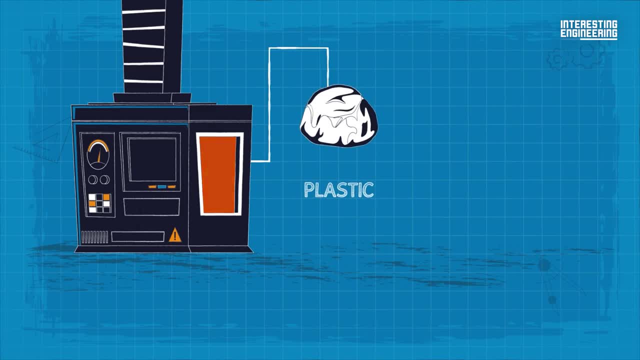 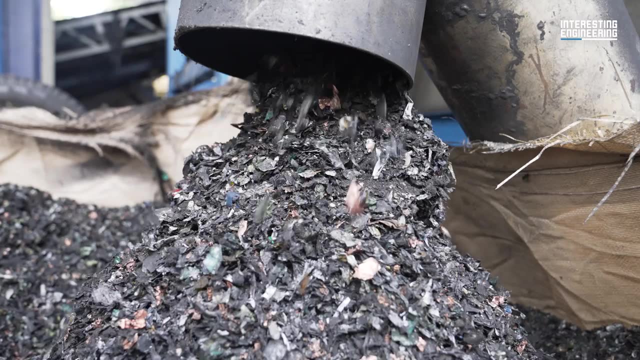 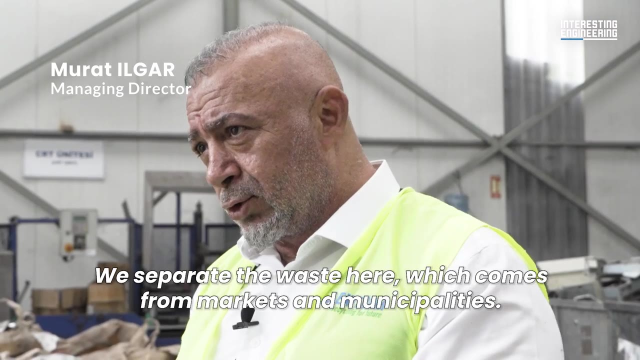 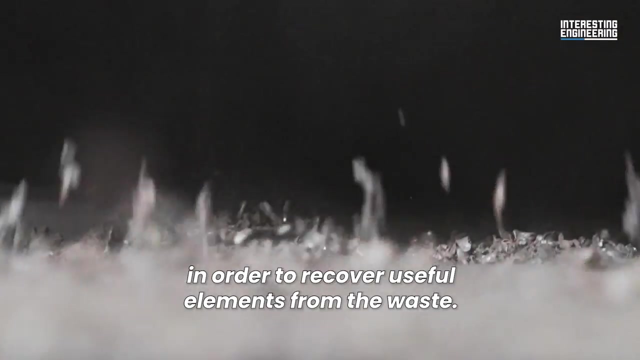 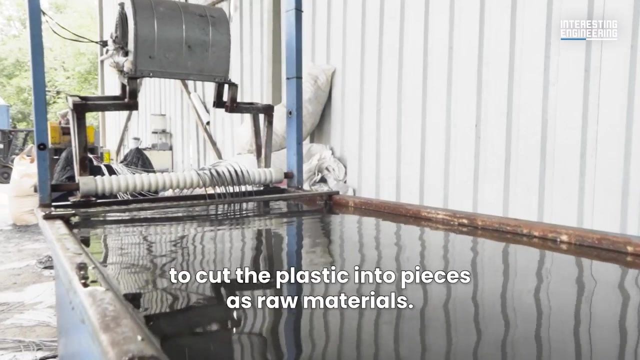 They apply heat to melt and separate the plastic, gold and plastic. They apply heat to melt and separate the plastic, gold and plastic. Then they control the metals and other metals from each other. wanted Both Doors. justification: after Butten Afterwood agua. 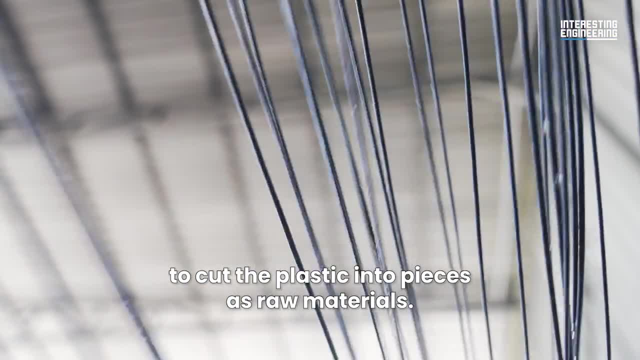 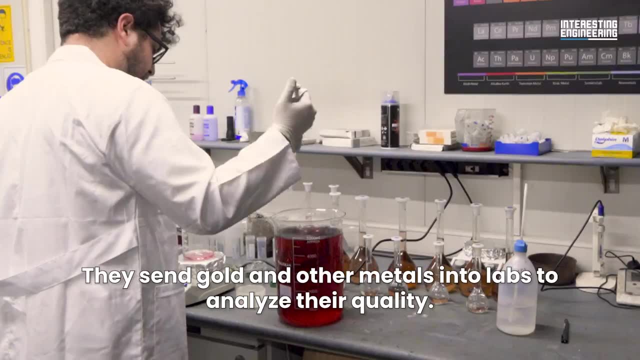 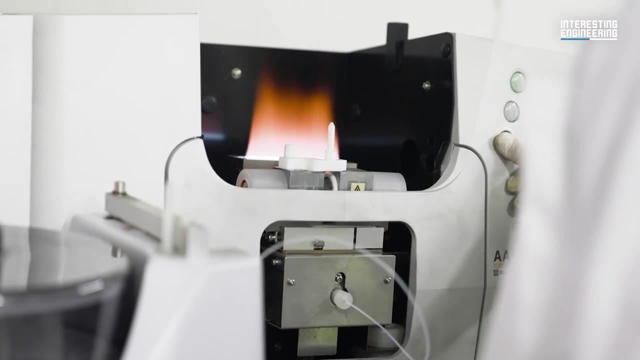 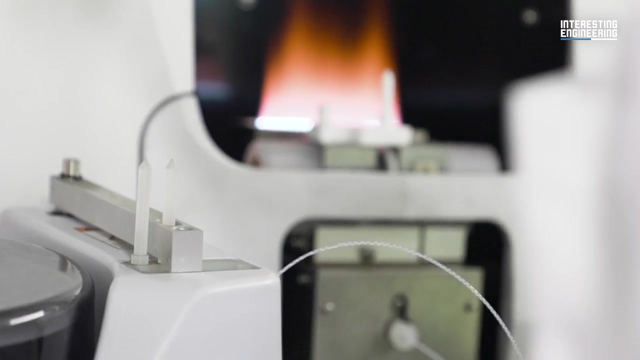 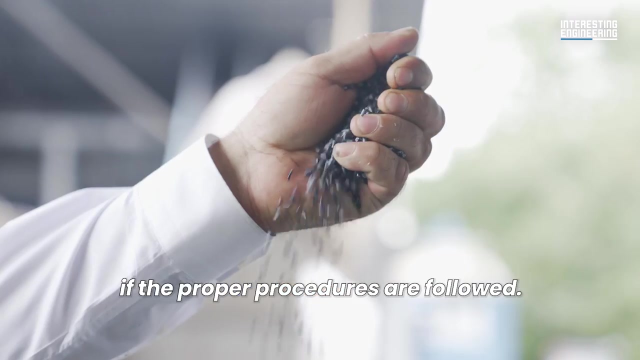 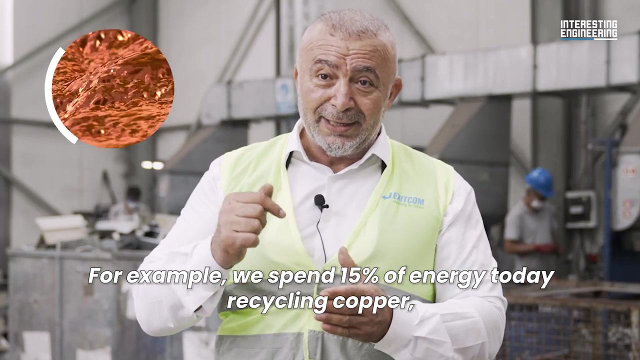 They put the molten products into cold water as raw materials. they send gold and other metals into labs to analyze their quality. That's what I'm talking about here. it's not just for the first time. If there are appropriate processes, all of these are recovered as raw materials. 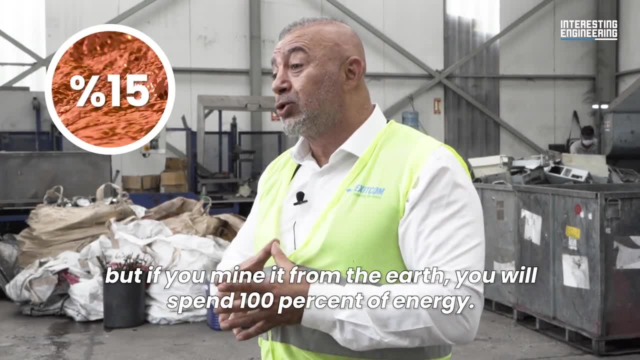 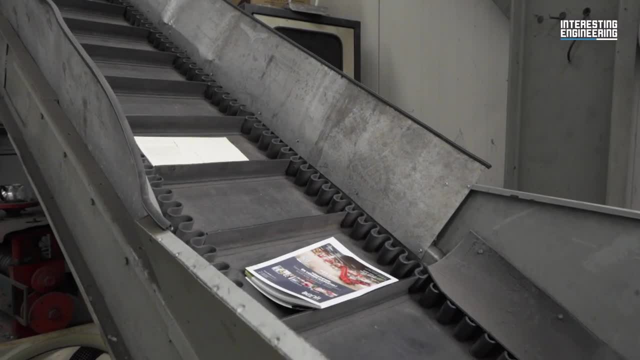 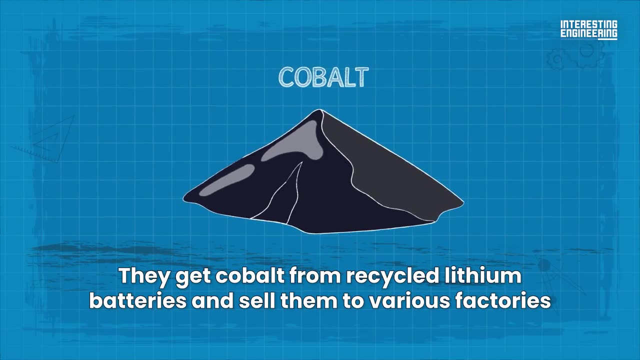 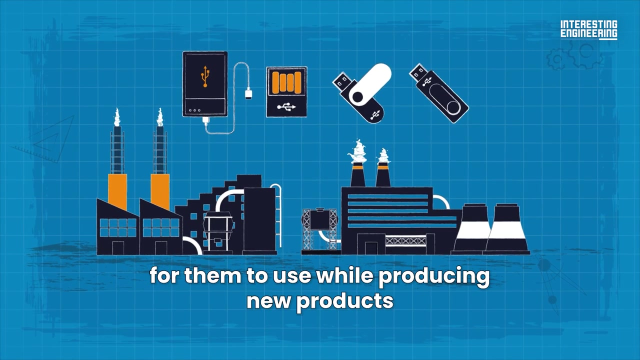 If you do a lot of recycling, you will reduce the nature again so much They use these materials as the feedstock of new products. They get cobalt from recycled lithium batteries and sell them to various factories for them to use while producing new products like magnets, stainless steel and storage devices. 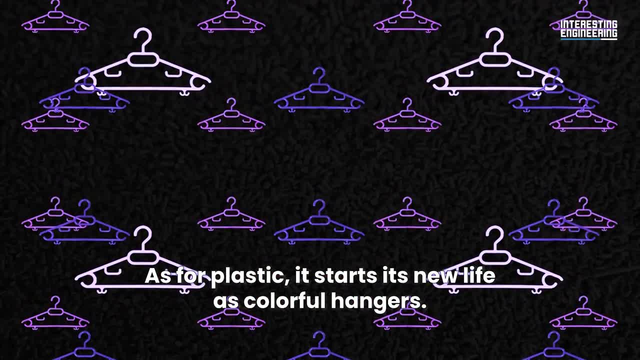 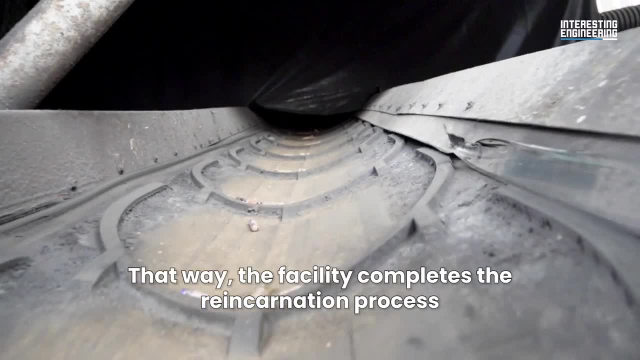 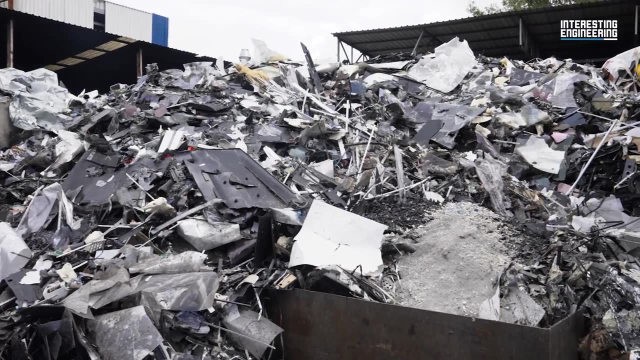 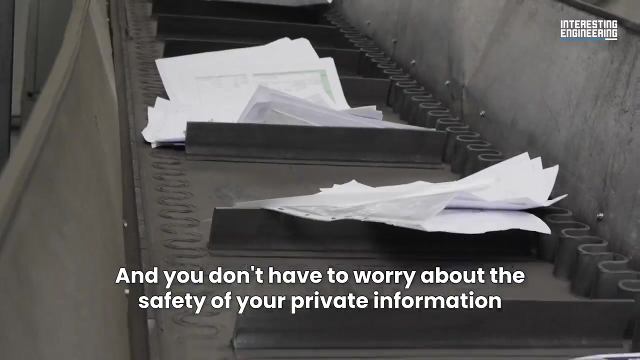 As for plastic, it starts its new life as colorful hangers. That way, the facility completes the reincarnation process and saves the planet from millions and millions of dead electronic waste. And you don't have to worry about the safety of your private information when you think. 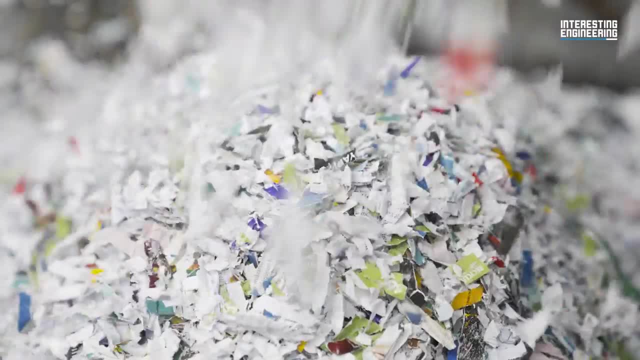 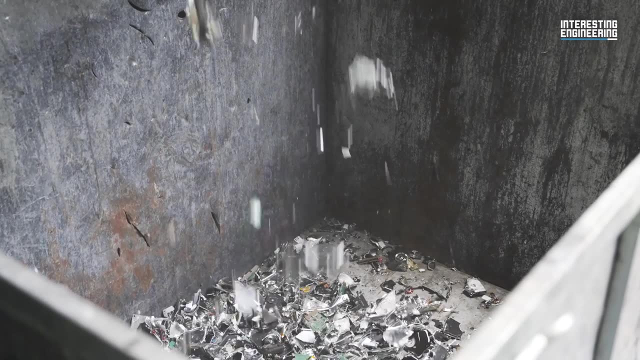 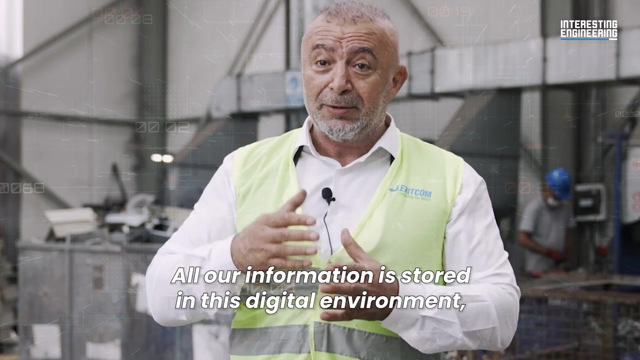 about your hard drives ending up in a facility like this, Because this facility also deletes and gets rid of this personal information beforehand. So they protect your privacy before they protect the environment. All of our information, our private information, the information of banks, the information of 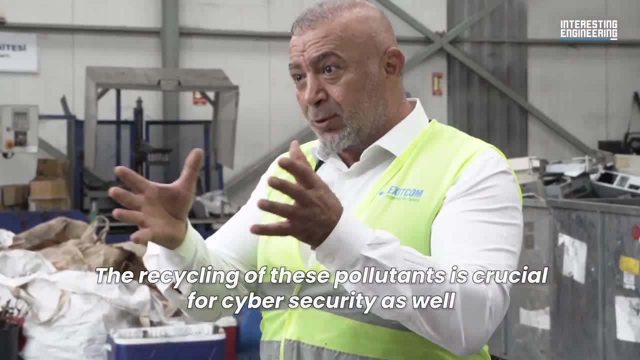 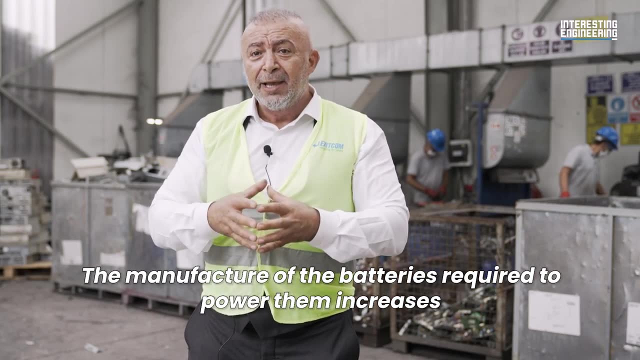 the state. all of this is in this digital environment. Once again, in terms of cyber security, in terms of digital security, these waste should be returned in this way Again, the raw materials in this, for example, batteries in the world right now, you know.